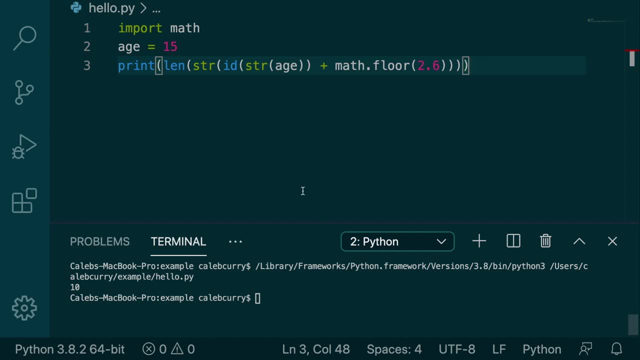 when we have nested parentheses. so anytime we have parentheses like this, the thing in the most inner parentheses happens first. So let's take a look at our expression here and try to figure out what's going on. And we'll start here, on the left side of this, plus starting with this age. 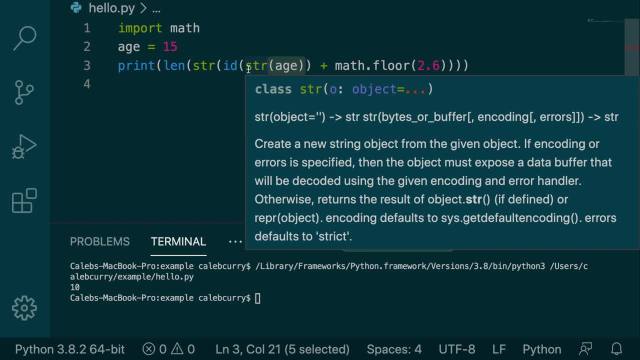 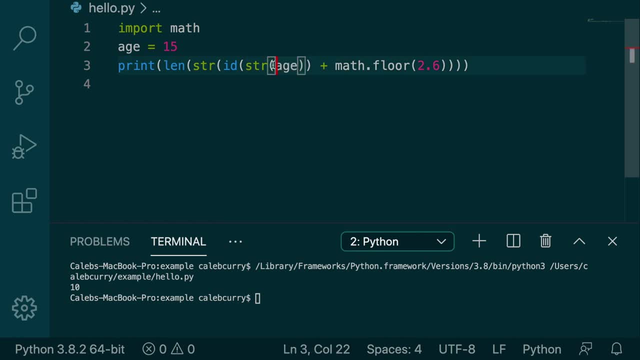 here. And when we pass something to this string, it creates a new string object from the given object. So this age 15 is converted to a string. And when we pass something to this string, it creates a new string object from the given object. So this age 15 is converted to a string. So these 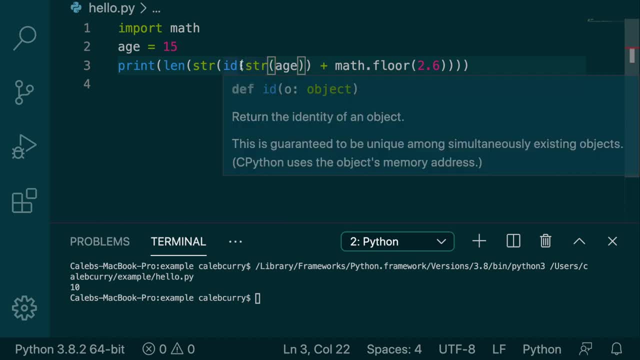 parentheses are for the string call, Then these outer parentheses are for this ID call, which is a function we talked about that returns the identity of an object. And then, lastly, we have these parentheses here, which includes this plus operation: mathfloor 2.6.. Once those two numbers are added, 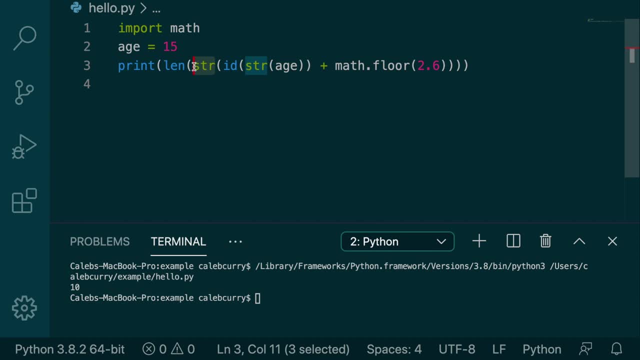 together. they are converted to a string, which is then passed to the length function, which is then passed to the length function, And then we pass something to this string, which is then passed to the print function. So if you needed to break this out into the steps, it's going to look something. 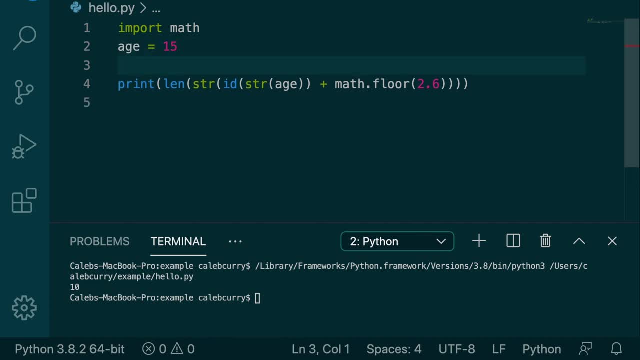 like this: So we have the age and then we convert that to a string, So we pass age in and this is going to be age string, just for we're going to need a bunch of variables here, So just follow along here. So that was the first thing we did, And then we got the ID of the age string. So that's. 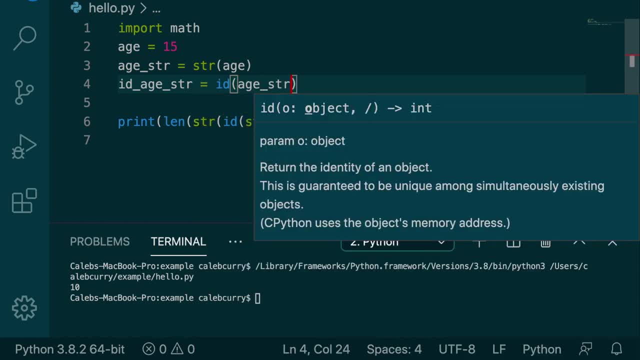 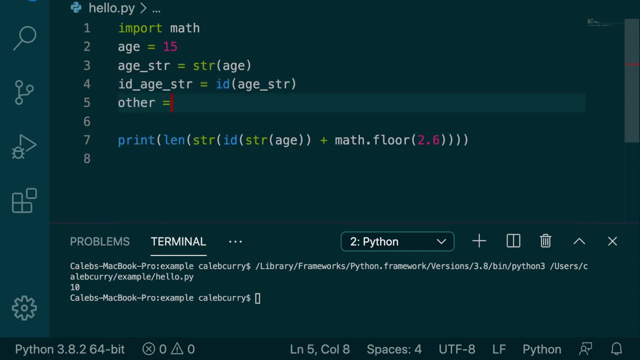 going to be ID of age underscore string, Then that whole thing is added with the mathfloor. so we could just create another variable, other and say mathfloor passing 2.6. add those up So we'll say ID age of string plus other. that gets passed to string. So one more time we will say added. 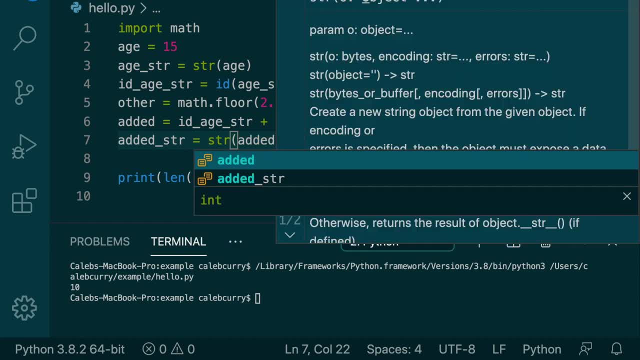 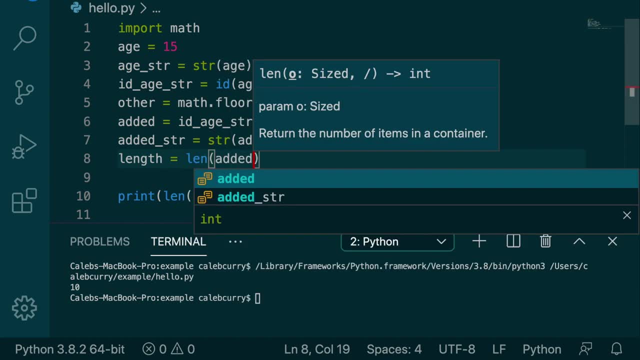 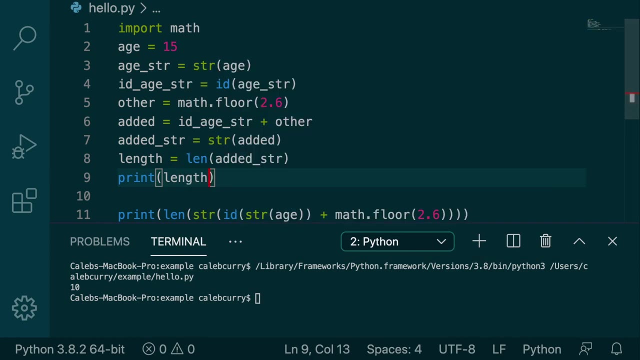 underscore string and then pass that in like so, And then we get the length of that Like so, And then, lastly, we print that. So we say print and we pass in length like so. Oh, okay, running that. 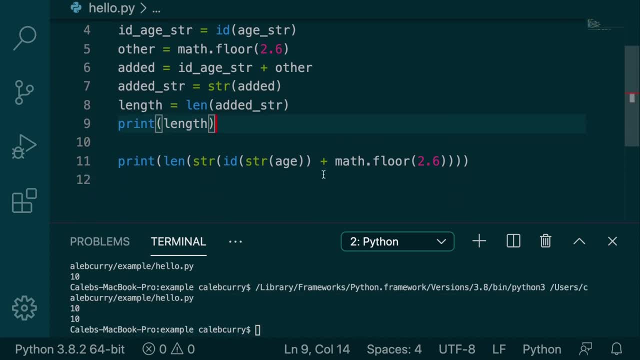 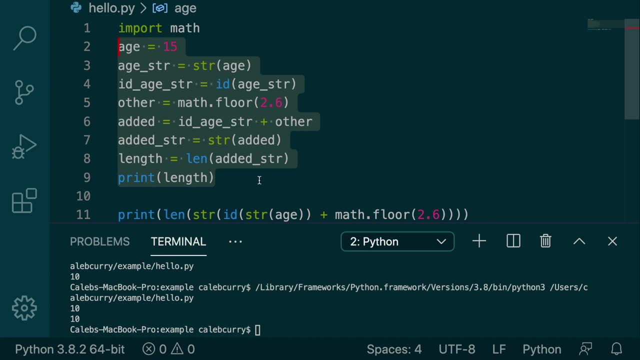 we get the same exact value. So you can see how nesting is actually a lot cleaner, Because this reading this, there's so many different variables And it would be really hard to go through this and follow, Although you can see step by step what happens. But this is a little bit more concise.